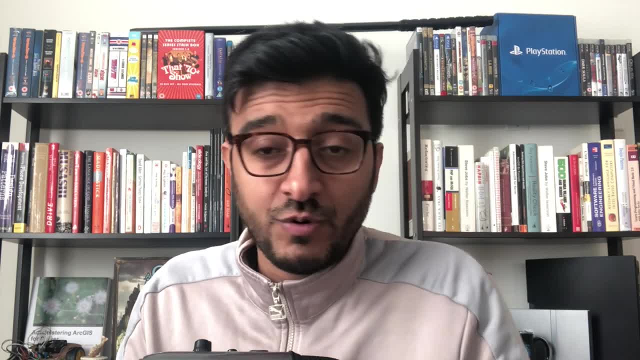 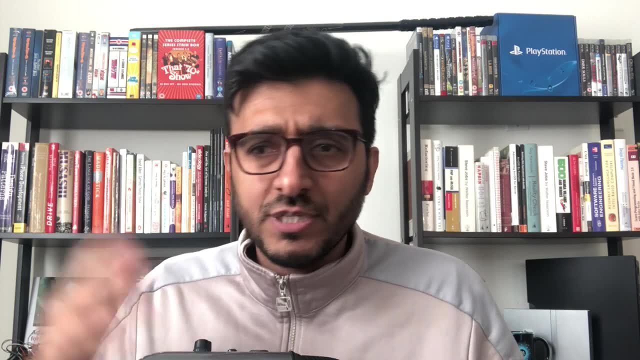 In this video I'll explain three types of caches that you can use in your backend application to improve the performance. If you're interested, stay tuned. What's going on, guys? my name is Hussein and I discuss backend engineering in this channel, mainly If you're interested in stuff. 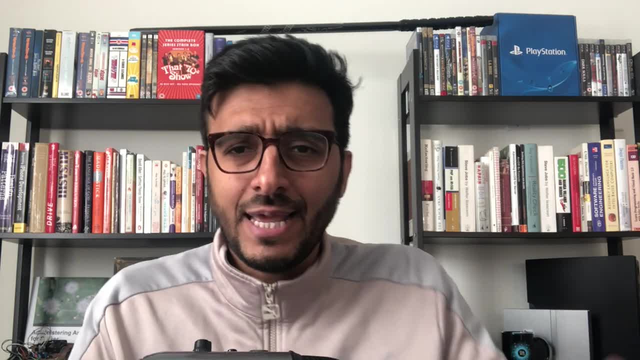 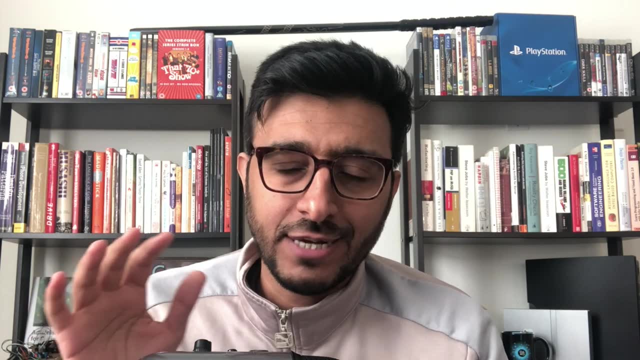 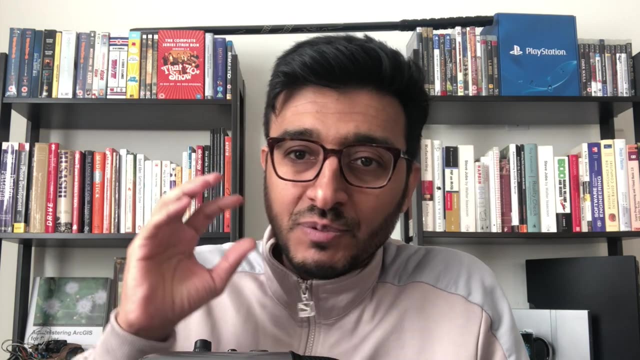 check out the other content of this channel. subscribe, hit that like button and let's just jump into it. So the idea of introducing a caching mechanism or caching layer in your app is because the mechanism or the cost of obtaining a certain amount of data is costly, is high. You want to. 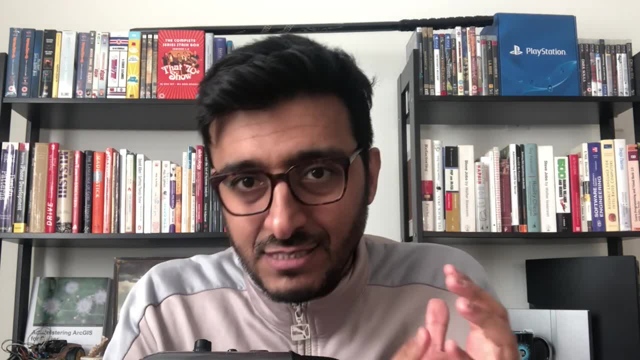 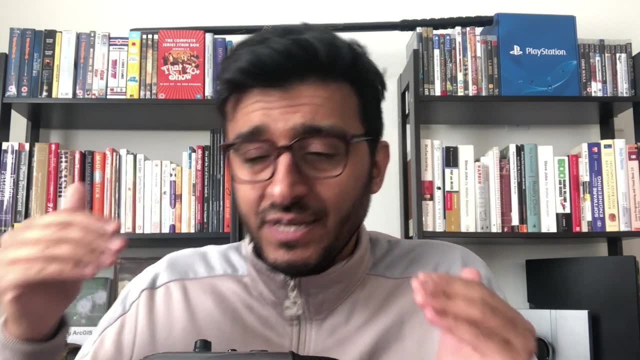 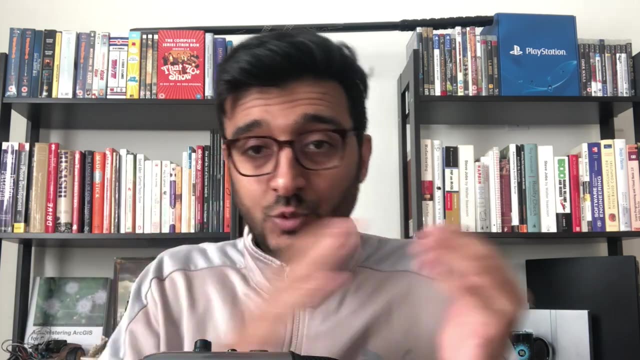 introduce a backup, fast access, so you don't have to go every time through the slow storage. And that could be in case of a database disk, right, Whether this is hard drive or SSD and you want to replace it with memory, or in case of CPU. The CPU builder build the cache so that memory. they want to avoid memory access because to them memory access is slower than actual actual register caching layer in the CPU. So we want the goal of having a cache is to avoid the extra cost of going to obtain certain information. So that's. 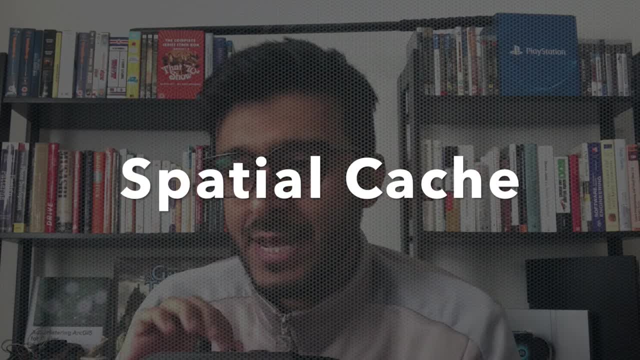 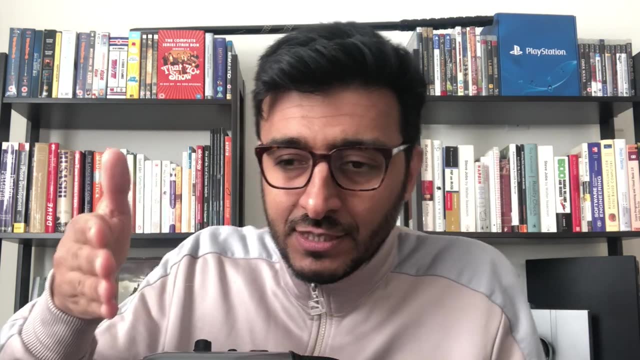 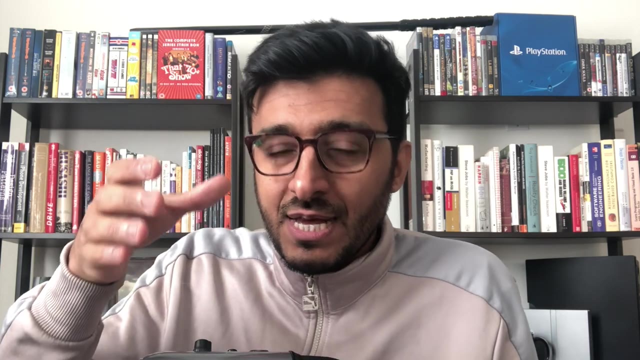 caching. So the first type of caching is called a spatial cache. And think of. a spatial cache is a locality based cache. That means here, hey, you're going to the desk And you are pulling a certain block of data. A spatial cache is: 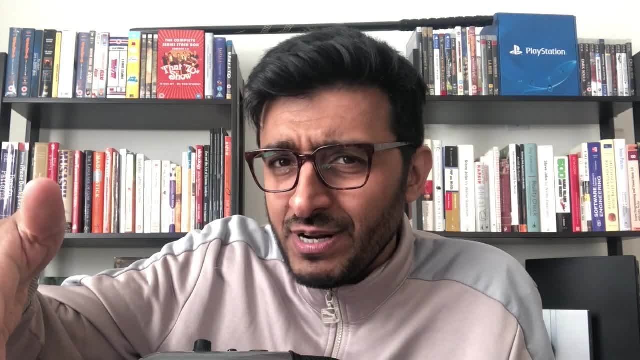 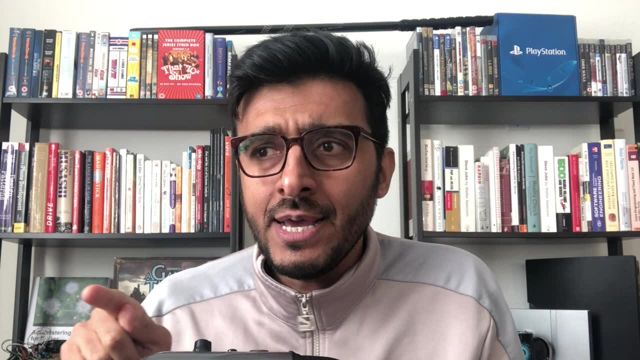 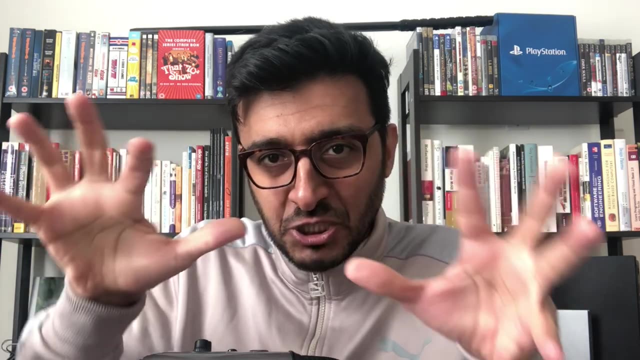 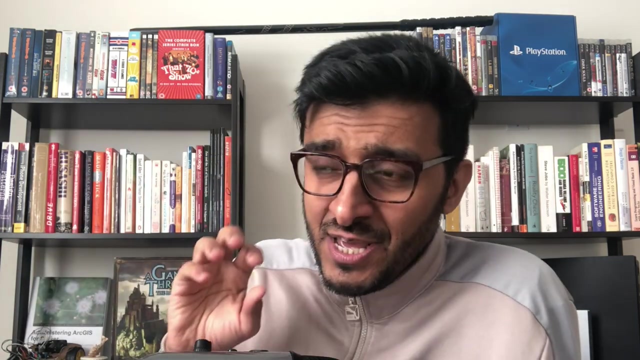 thinking the Apple thinks is: hey, since I am already took the hit and did that IO, might as well let me get the nearby blocks, because I am predicting that a future request will need this spatially located blocks or spatially located data. So that's called spatial cache. So that means if I'm going there, 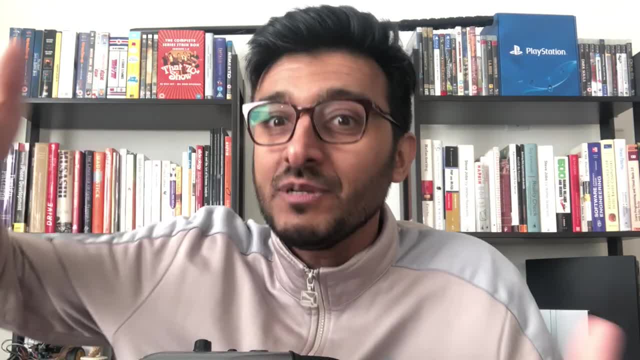 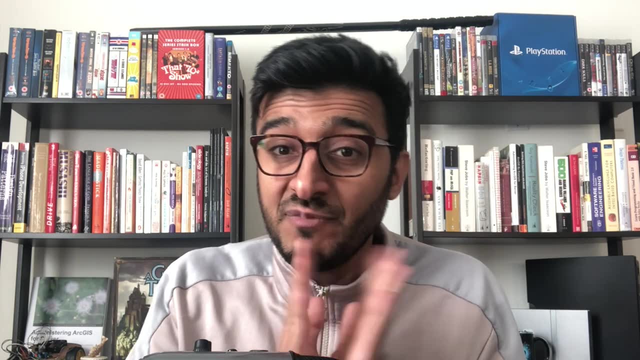 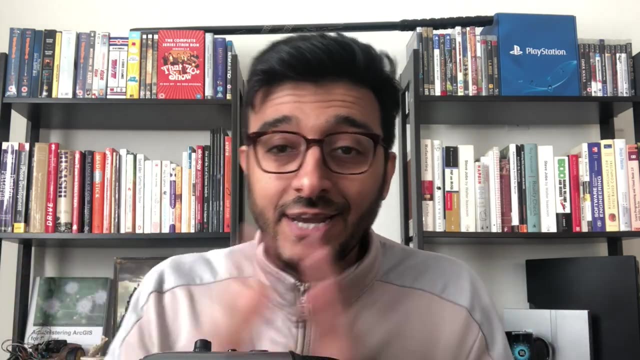 might as well just pull this stuff, so that I already took the head. let me pull nearby located data so that in future requests, if they requested this data, they can benefit of this Usually. one example I'd like to think is like if I am assembling a table from IKEA, right and and, and I am assembling it upstairs and all my 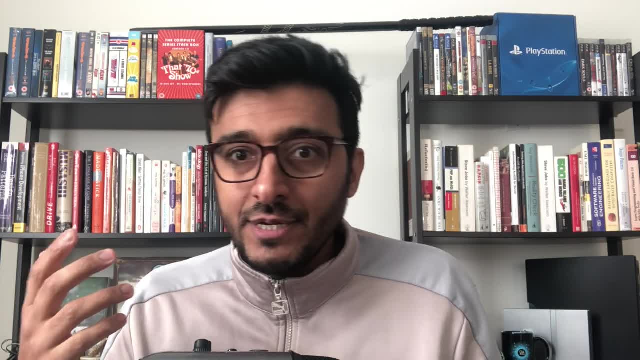 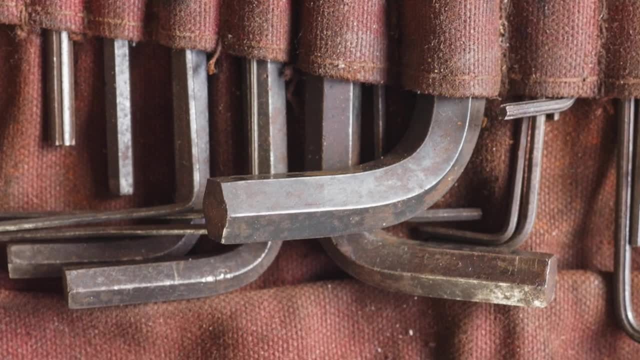 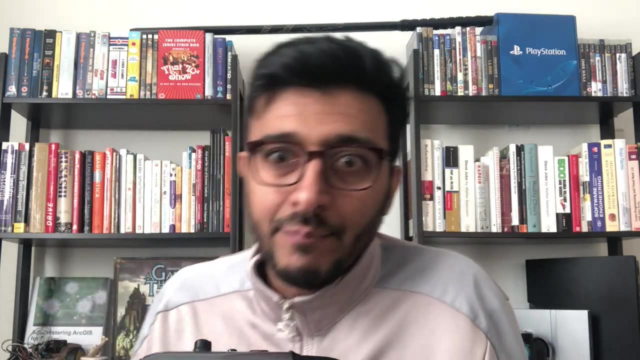 equipments are downstairs right and all of a sudden I need a screwdriver. So I go down and pick up a screwdriver and go up, And then, while working, oh I need an Allen wrench. this, this, this weirdly weird thing- that hexagon looking right wrench. So let me go down and pick up, pick it up. 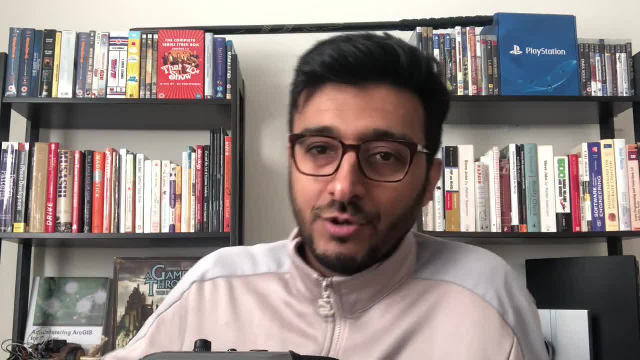 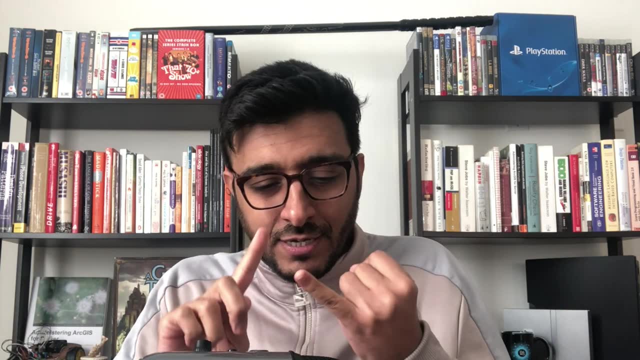 again And then, oh, I need a drill, Now, let me go down and pick it up. So if I am smart enough and say, Okay, let me look at this table Now. I'm going to need an Allen wrench, I'm going to know a screwdriver and I'm going to need a drill. So let me go once. 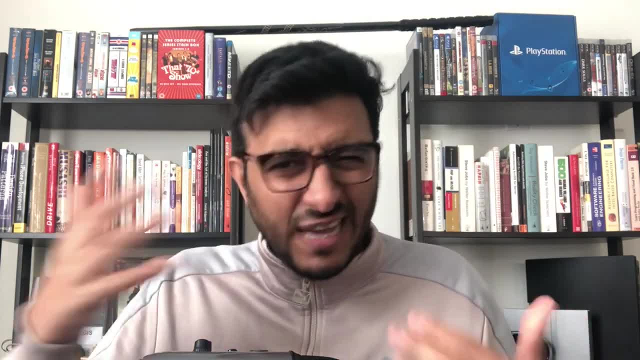 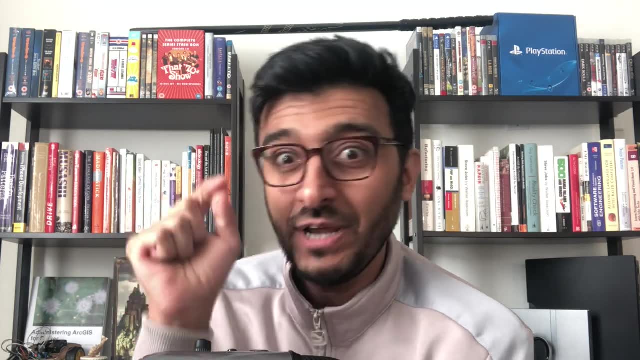 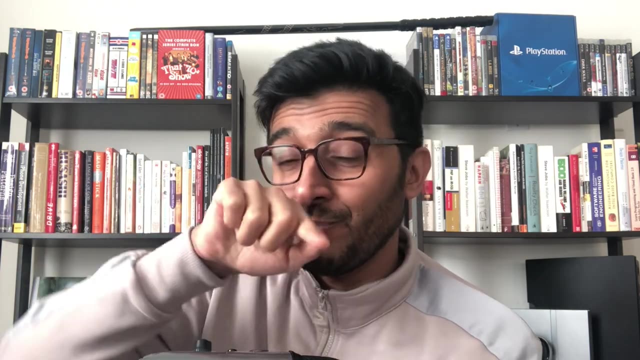 downstairs, pick up all this stuff and then work on them. So that's an idea. So the trick here is: if your back end app can actually predict what is going to need- and that's not necessarily easy by any chance- then it's going to be useful to pull up. 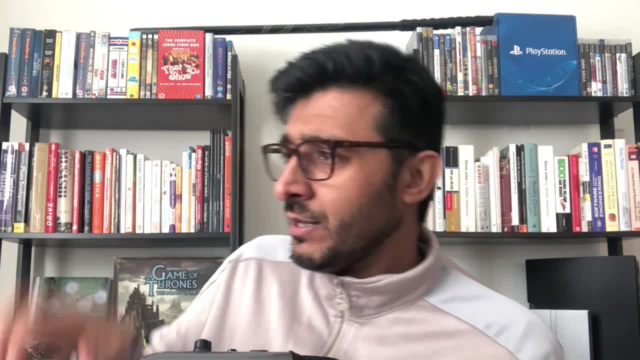 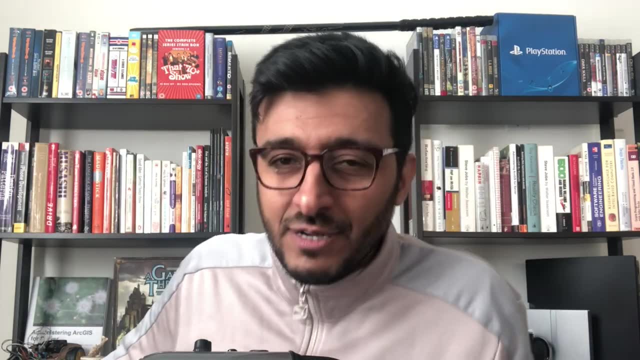 spatially located things. So when I went back down, oh, here's the screwdriver, Since I'm gonna let me get the drill. it's all located, spatially located. So that's the idea here. Alright, so that's the first cache spatial. 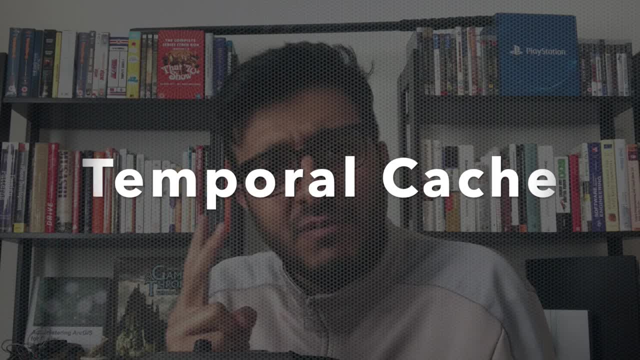 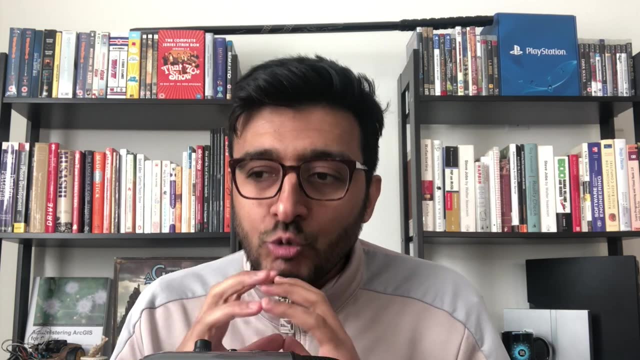 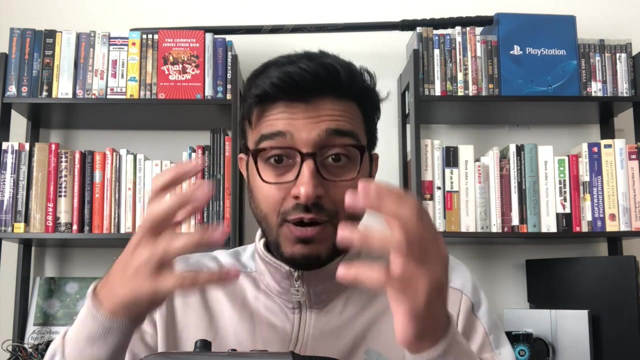 spatial cache. The second type of cache is called temporal cache And that's relative to time. So most most frequently used here is I am. I went there and I pulled a piece of data, okay, And now I cached it. And now you start caching other pieces of. 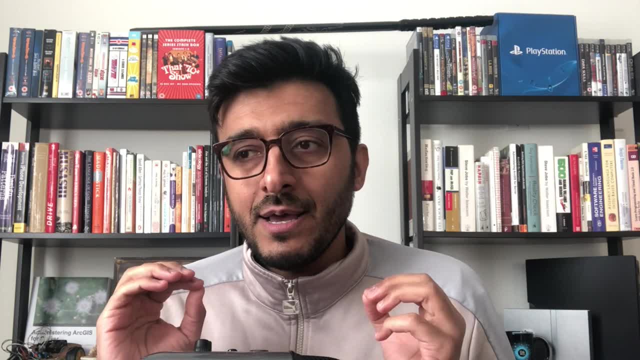 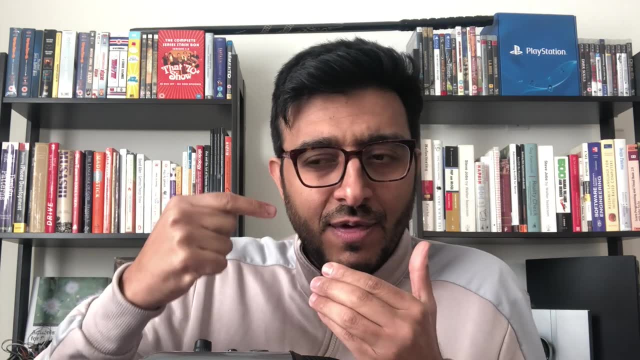 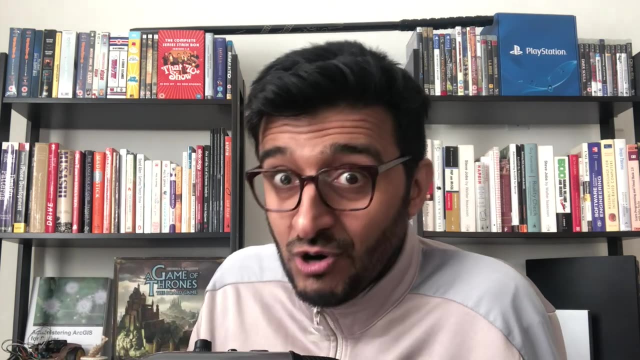 data. If I I asked for a certain piece of data that is available in my cache, then the the most frequent access data are getting hot in the cache. they are not discarded, So that's called also a least recently used cache, where where the least recently used cache are. 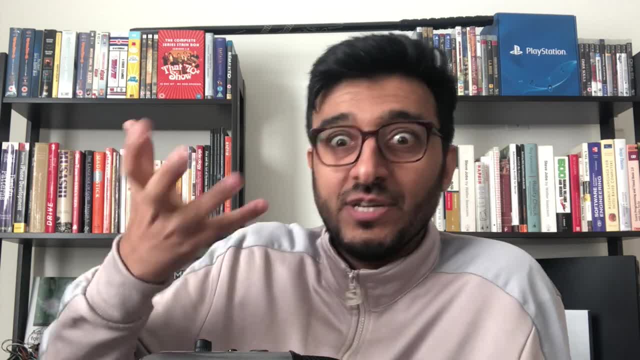 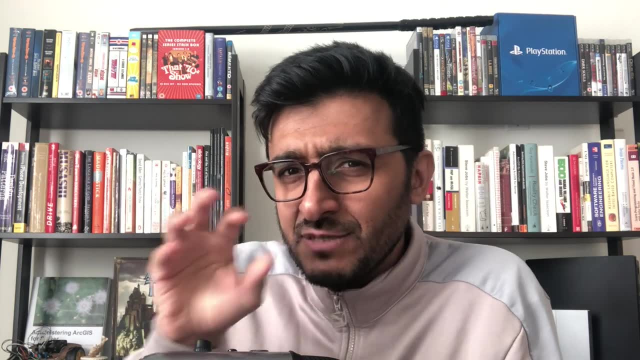 getting thrown away, while the most recently used cache is getting bubbled up right. So that's, that's the idea of a temporal cache. So if you're using a piece of data a lot, then you're probably going to use it in the future. So you keep it fresh in in the 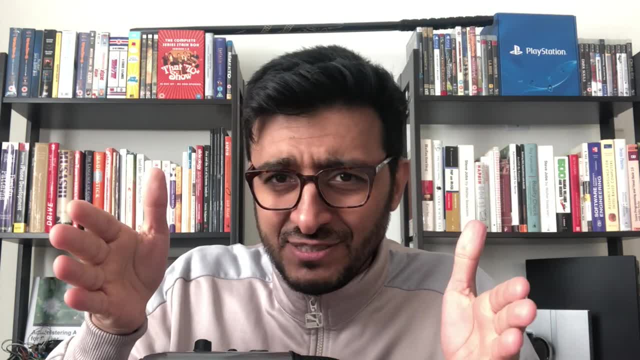 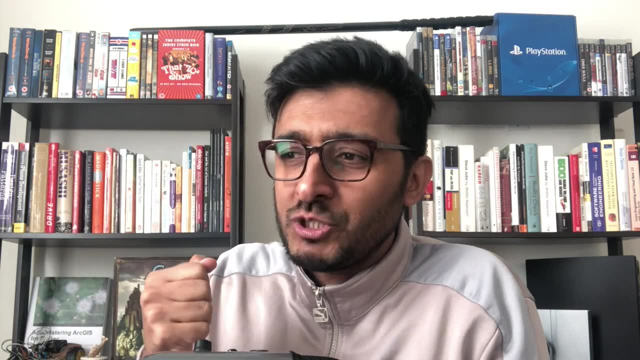 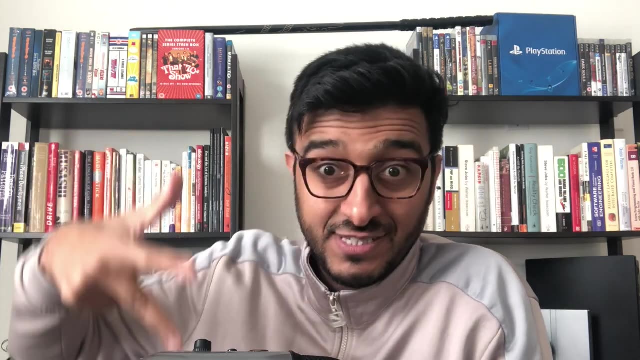 cache, because the cache is going to be only limited, right, It's not going to be infinite, Otherwise our all problems will be solved, right. So that's, that's, that's one approach. Actually, the CPU uses where L1 cache, L2 cache, L3 cache, where this is actually a 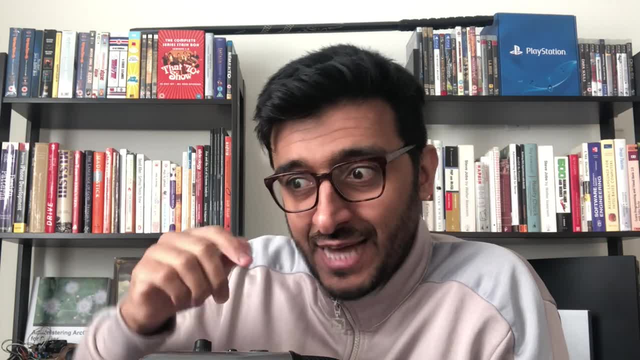 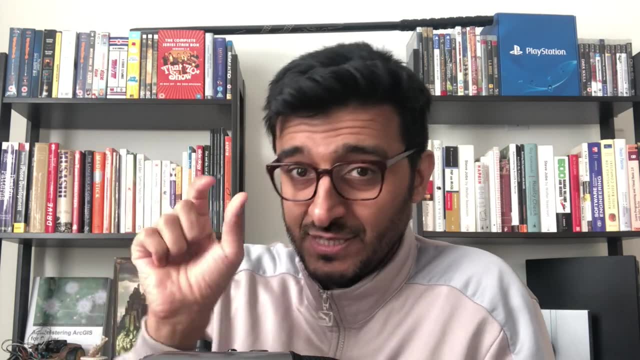 temporal cache where, if it's a, if it's frequently asked, is going to jump to the faster cache. I forgot which the faster cache is the L1 or three. it's going to pass to the faster cache, the smaller one, which is the faster access if it's not frequently used, going to bump them down all the way down. So 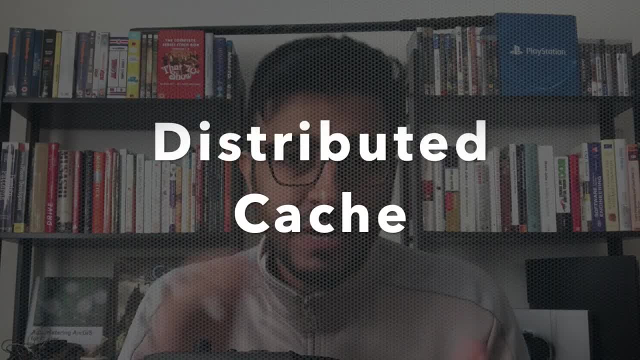 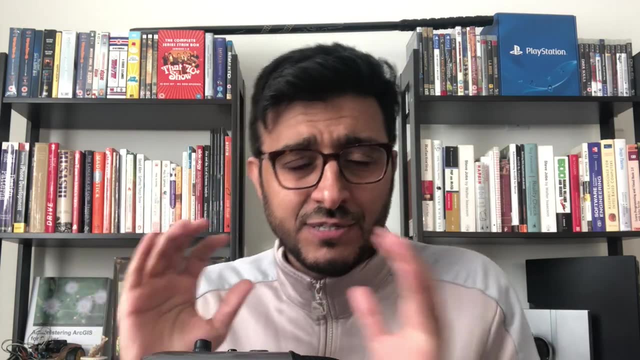 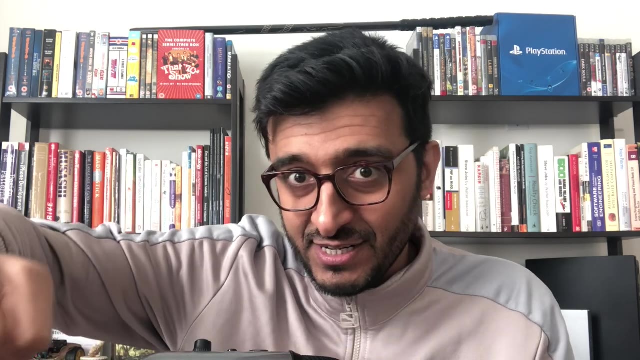 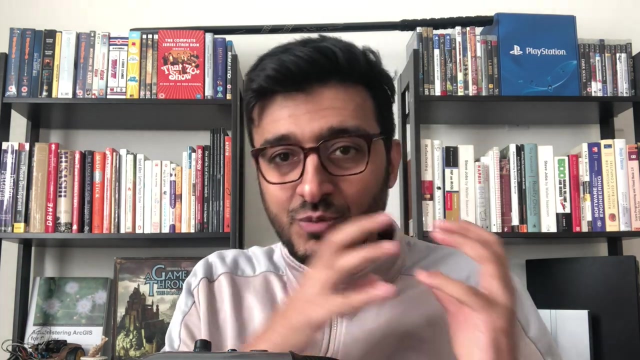 that's essentially the second type, temporal. So the third type of caching is called distributed caching, which is a combination of both, But that the trick here is you need to keep to keep cache in sync with the main data store, And most popular here is Redis. right, you have a central cache, Redis or memcached, And now when you, when, 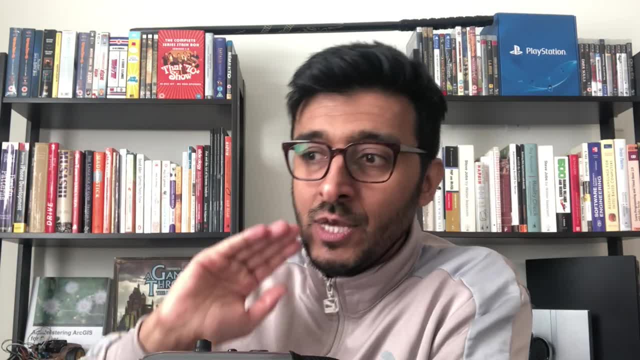 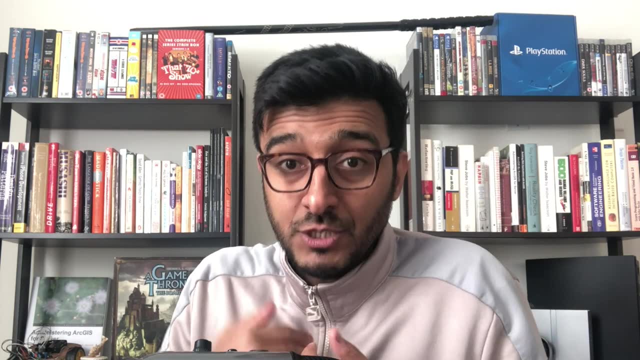 you want to read a piece of information, your cache is empty. you go to the disk and you pull a piece of info and then you populate the cache with it. So next time, if you want to read an information, you put ask Redis or ask your distributed cache. Hey, do I have this information? 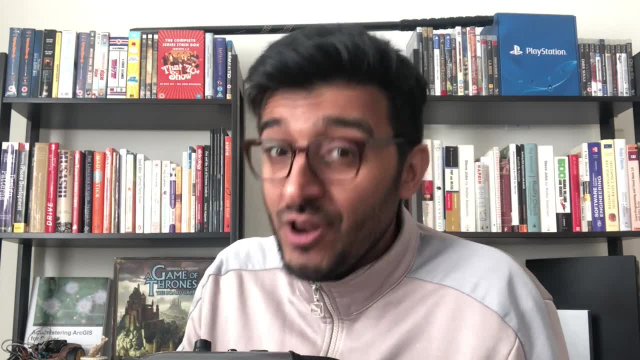 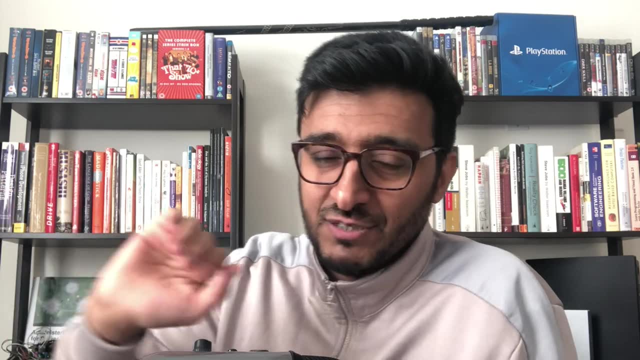 Yeah, yes, I do Here it is. No, I don't go to the disk Because, yeah, you don't have it, But that the disk must have it, right. So now it go to the disk and then pull it, And here's where it gets. 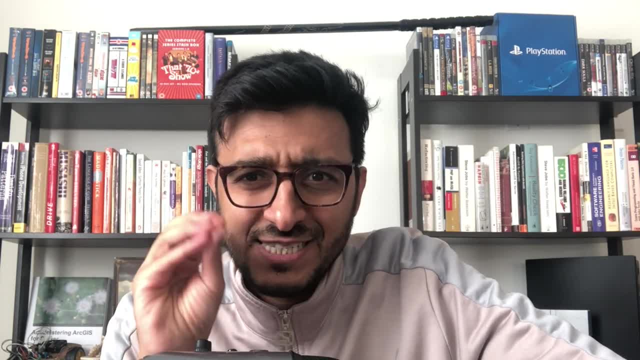 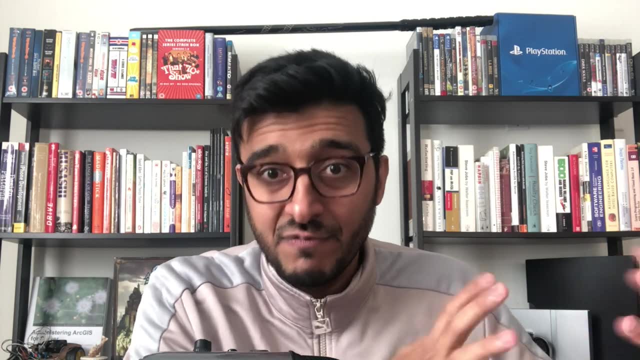 really tricky Because keeping the cache in sync with the main data store is one of the hardest problems that backend engineers face, and frontend engineers if they have similar cache in the frontend. So that's why there are two types of caching here And I'm going to make another. 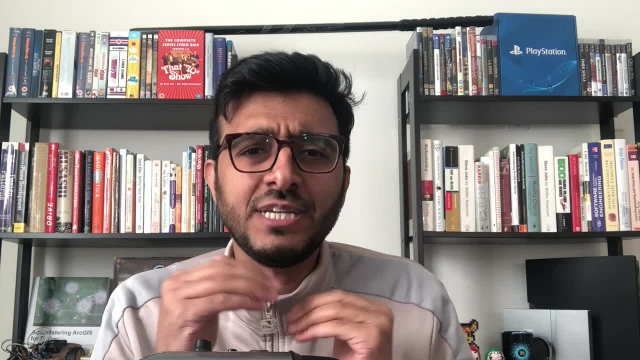 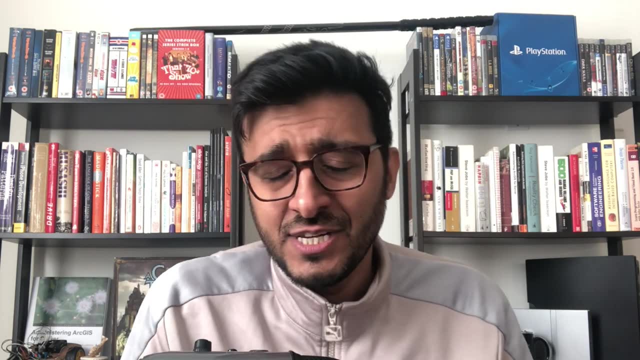 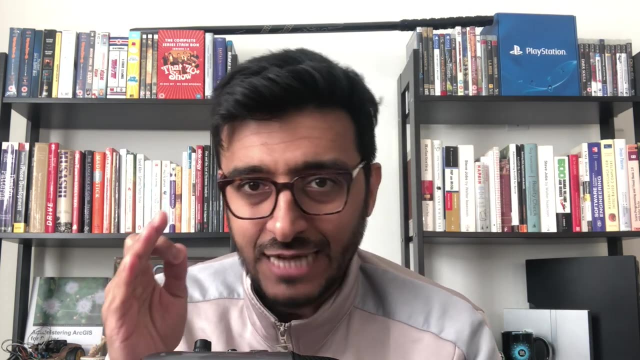 dedicated video for this. So this is especially when you're actually trying to write to disk and update your cache and keeping this cache in sync. So two methods so far we know about. There is one called write through cache where if you want to update your data store, you first do. 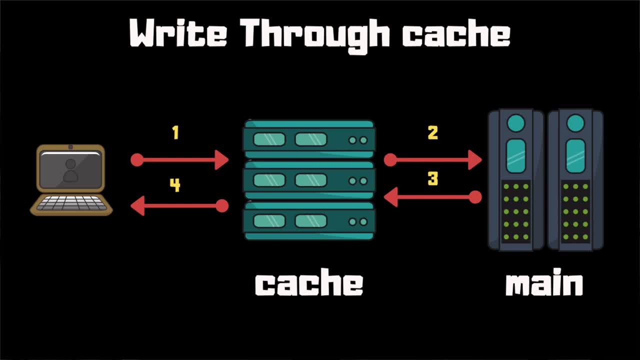 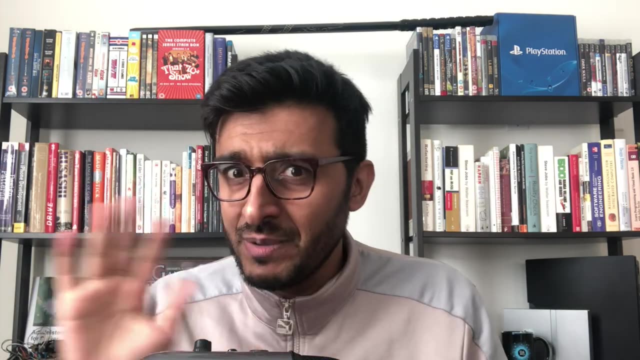 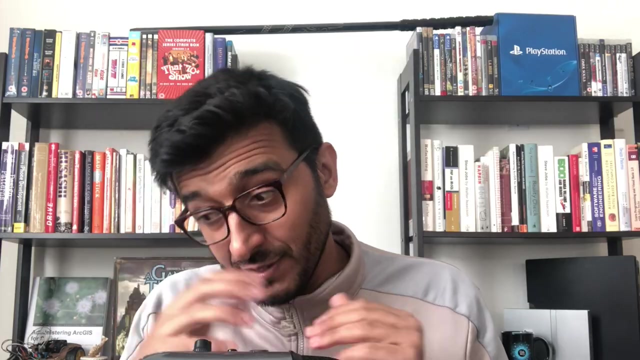 it in the cache itself. Ah, look at this. So you update your cache and synchronously block the client that is writing to write also to the to the IO disk immediately, right? So there are many implementation AWS doing differently. You can do it differently. So I know AWS have like a something called them. 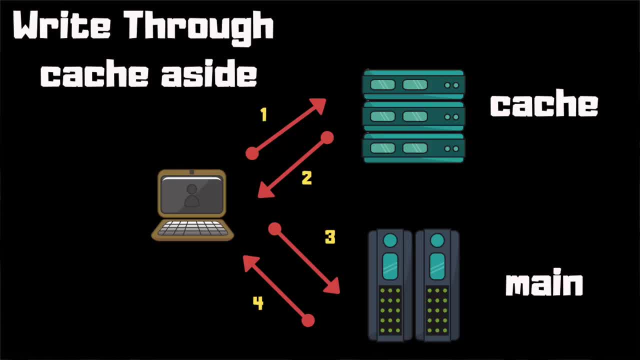 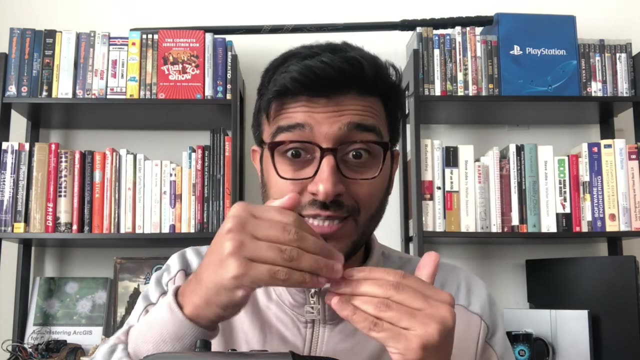 I think set aside or something like that, where the application is aware of both right, Just the write through cache, where the app writes to the cache and turn around and also write to the data store at the same time. So the app is aware there is another type of write through cache. 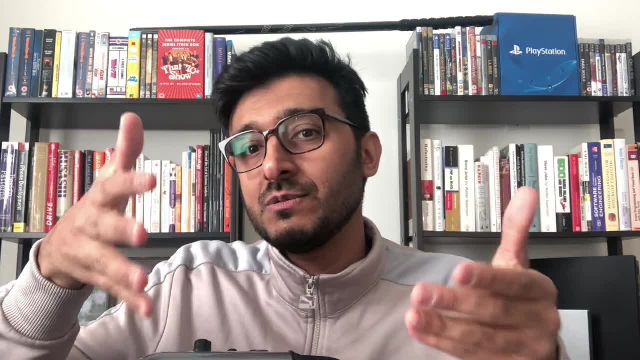 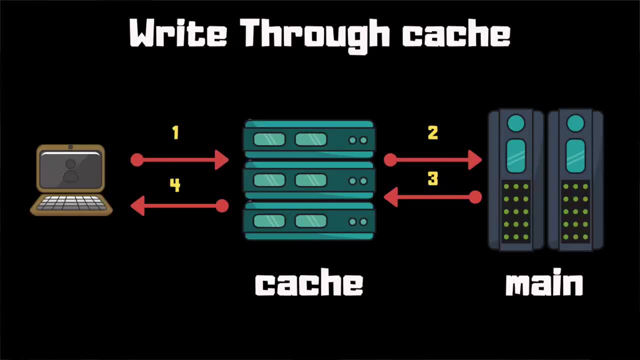 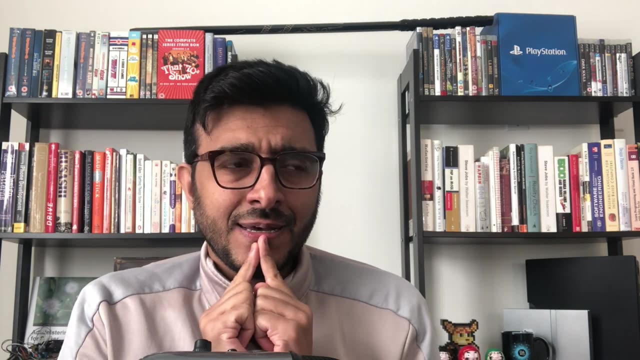 where you write to Redis or you write to this cache and you also synchronously block, but the cache turned around and actually writes to the disk. So it's, it's almost, as is, a true write through cache. This, this is the first type of write or write through cache, which is which is kind of nice, because now, if you 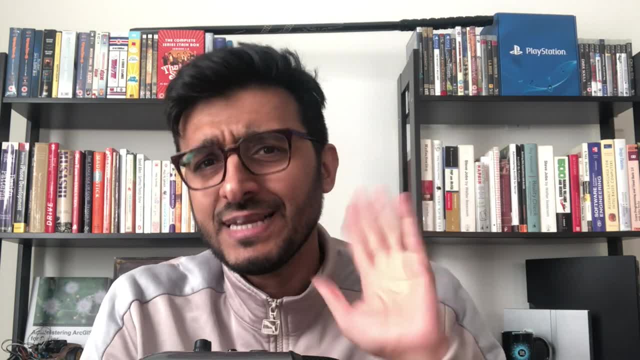 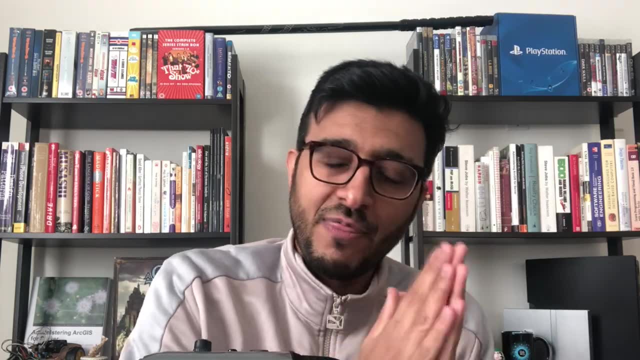 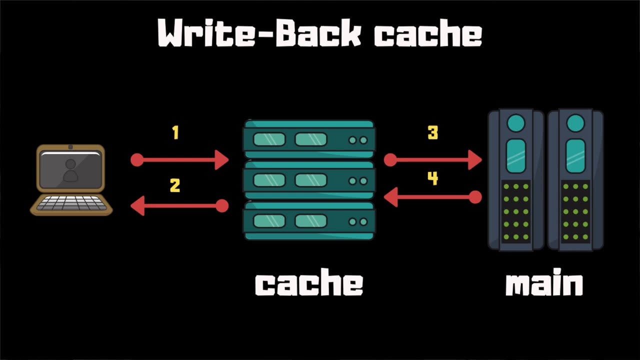 look, if you want to query, you always query the cache And you can guarantee almost that the cache is going to have all your data right, Because all the latest data the other type of the distributed cache that is called write back cache, which is almost asynchronous. So you write cache, you write to the cache and then 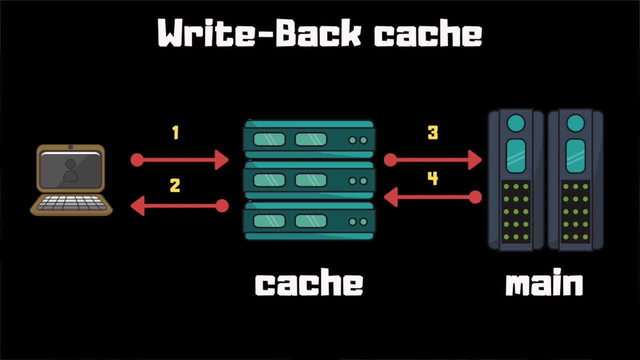 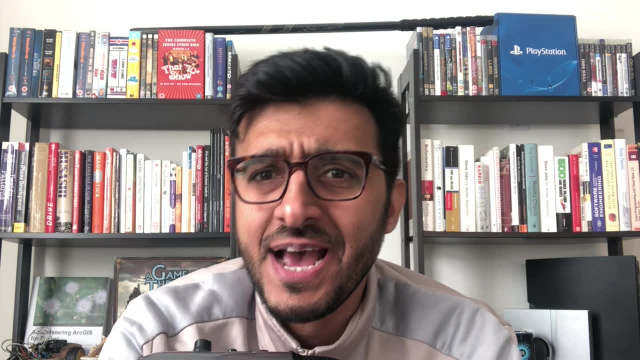 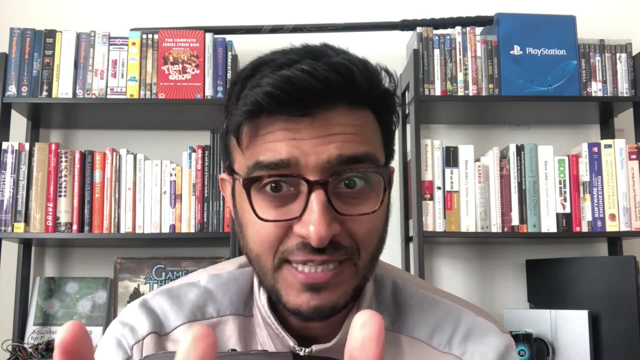 that's it. you trust that the cache you're done immediately There. the cache will asynchronously write back to the data store. A write back cache is way more complex to implement. That's the second type where essentially you're going to write- always to- 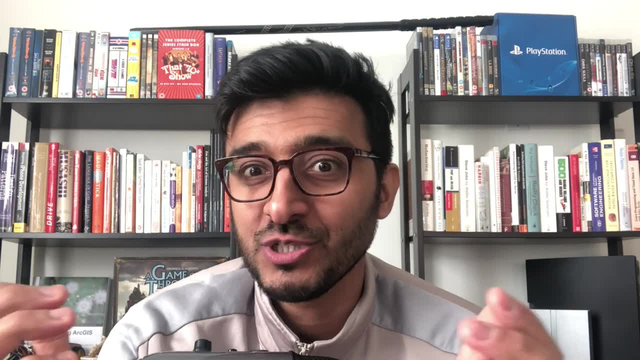 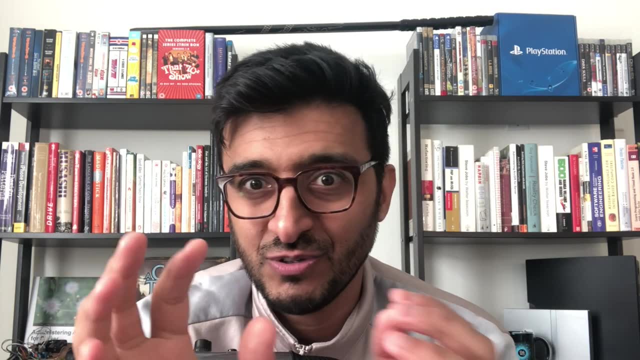 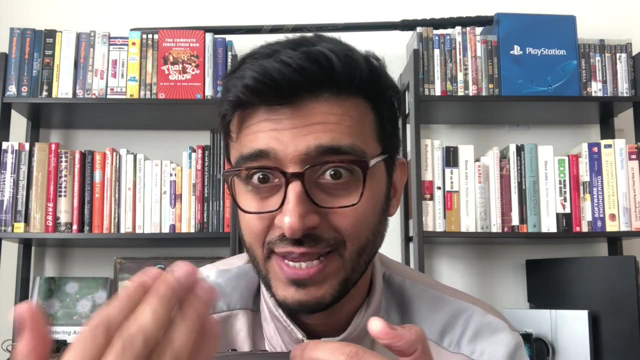 the cache. But once you write to the cache, you're essentially done. However, it's the cache store job to mark these pages or data that you just written in the cache as dirty as being edited. And now the cache is responsible to take all these dirty pages and then flushing that back. 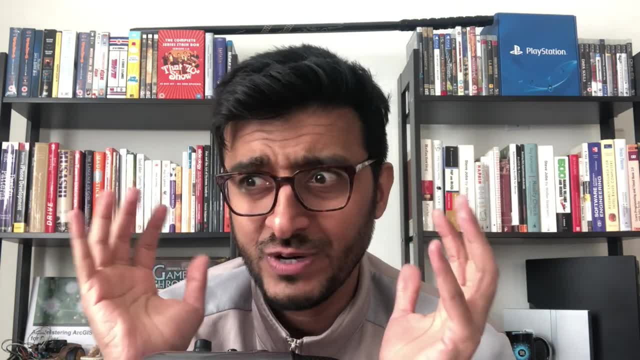 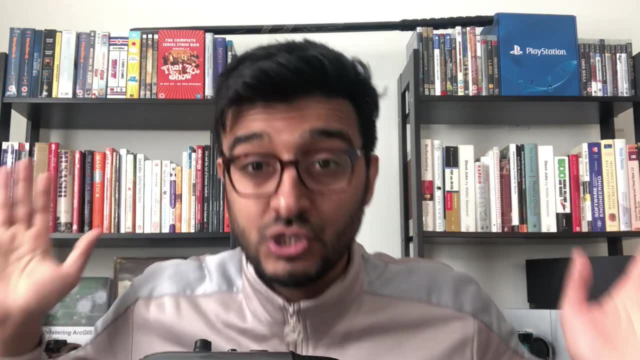 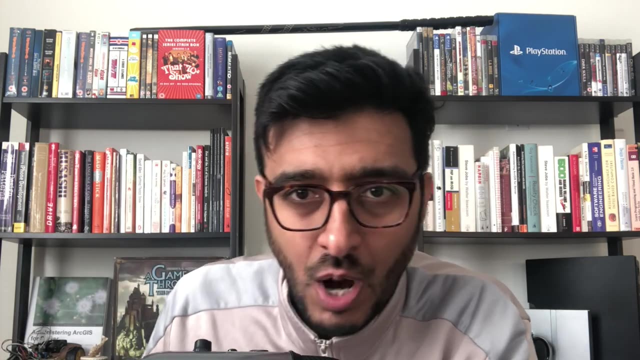 to the disk. Now there are lots of implementation where how can you guarantee persistence in this model? Because if you write to the cache and the cache destroyed in memory, that's a big problem. You just lost one of the asset properties, which is durability. It's not durable with write back. 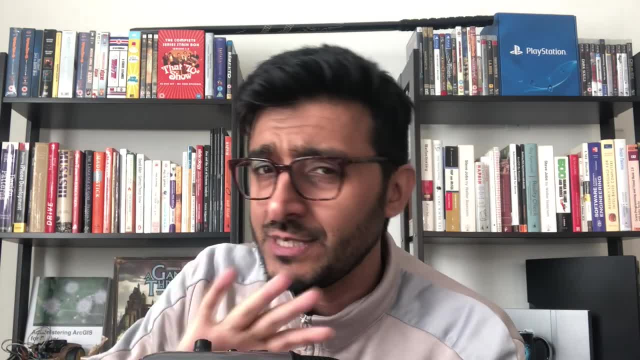 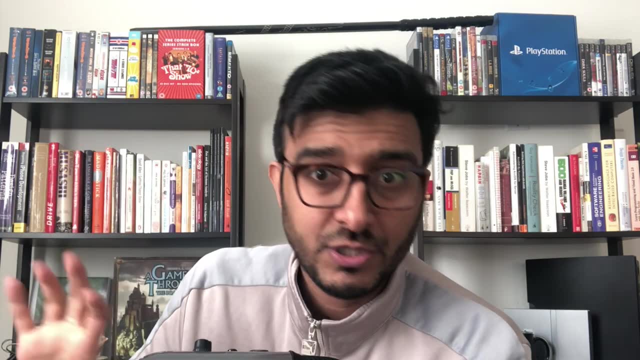 right. So that's one problem. Again, I'm not going to go into details about these two types. I'm going to dedicate to different videos specifically designed to talk about distributed caching and all this limitation, all that stuff. All right, guys, hope you learned a few things in this video, If you like this video. hit a like and I'm going to see you in the next one. You guys stay awesome, Goodbye.